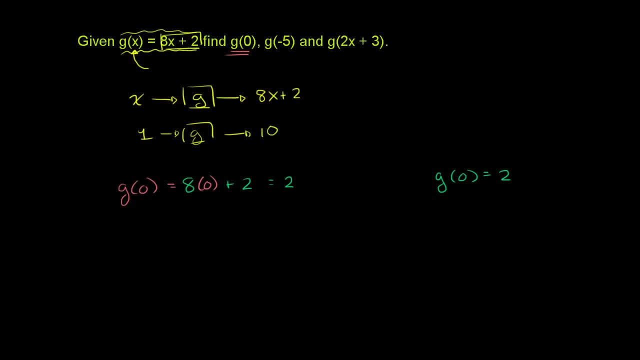 Let me just write that here g of 0 is equal to 2.. Now let's try g of negative 5.. So let me write it this way: g of negative 5 is equal to- and I'll try to do the color coding a little bit better this time. 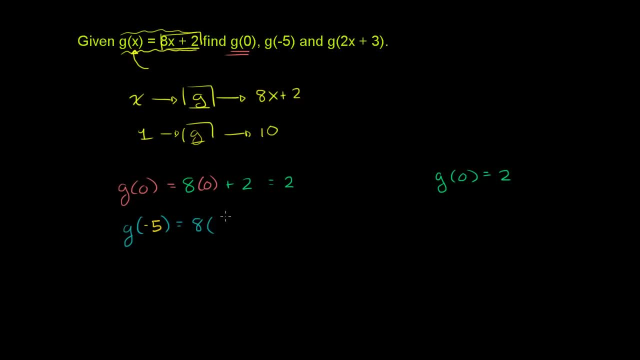 it's going to be equal to 8 times our x, which in this case is negative 5,, 8 times negative 5 plus 2.. We're inputting a negative 5, and we're going to output 8 times negative 5 plus 2.. 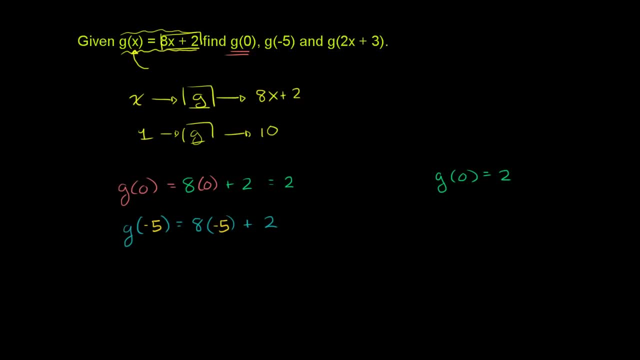 Wherever we saw the x, we just replaced it with a negative 5.. And this is just equal to 8 times the negative. 5 is negative. 40 plus 2 is equal to negative 5.. So I'm going to write this over here. on the right: 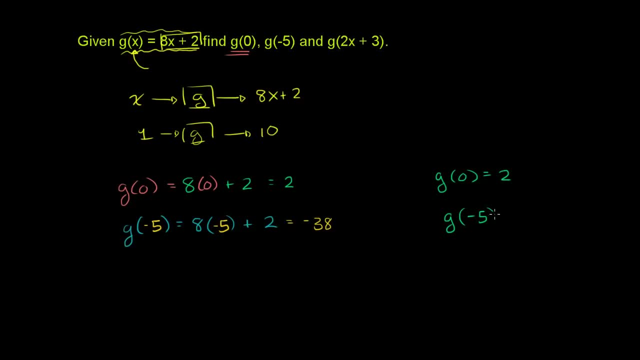 We have g of negative. 5 is equal to negative 38. Now this last one is a little bit interesting, So we just did this one. Now let's do g of 2x plus 3.. So now they're not inputting a number. 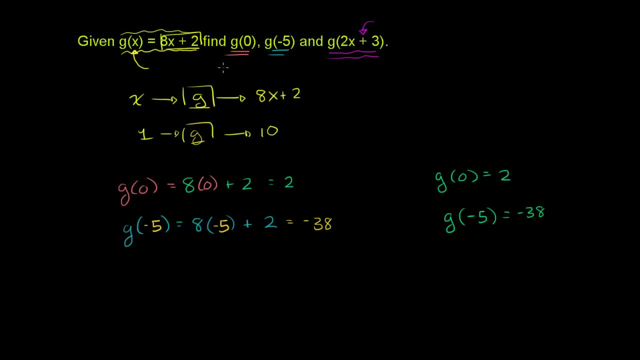 They're inputting an expression And what we have to do is, everywhere where we see x here, we're going to replace it with that expression. If I did g of a circle, let me write this down: I'm going to write g of a circle. 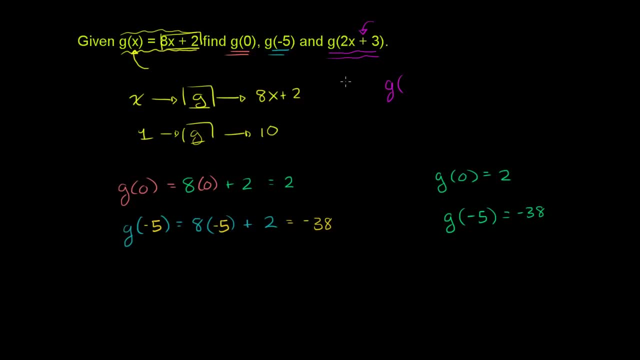 Let me write this down. I'm going to write g of a circle. Let me write this down. Let me write this down. Let me write this down: If I did g of an orange circle right over here by this function definition, if I'm 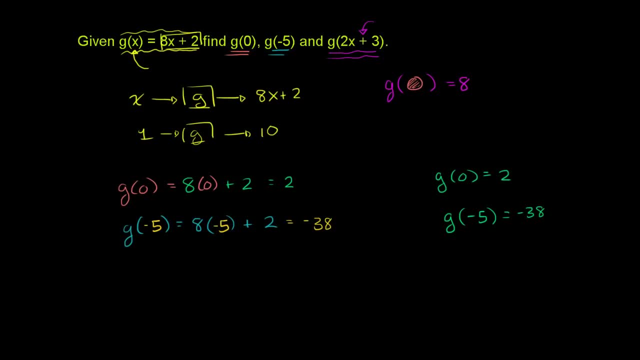 inputting an orange circle. I should output an orange circle 8 times the orange circle, which doesn't make a lot of sense, But hopefully you get the idea that whatever you're inputting, you're just going to multiply it times 8 and add 2.. 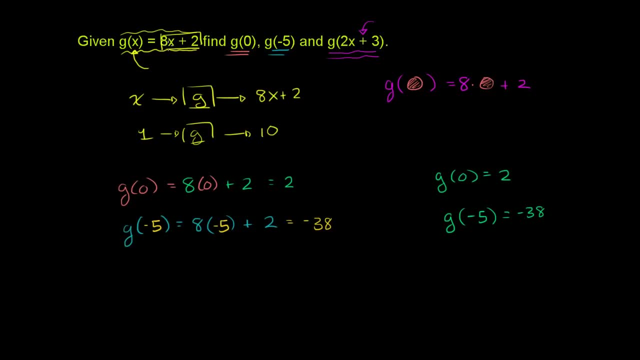 So if we input 2x plus 3, we're going to output this times 8 plus 2, wherever we see an x, we replace it with this right over here. So let's try that out. So now we have g of 2x plus 3 is going.